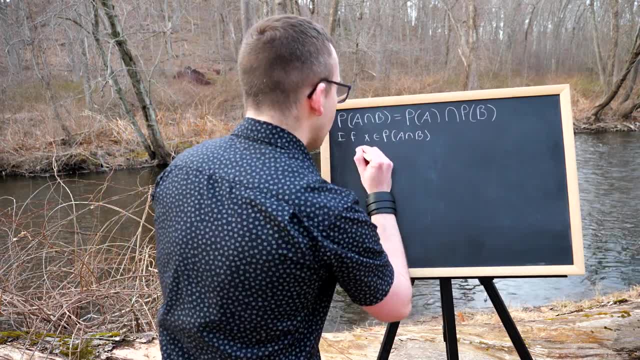 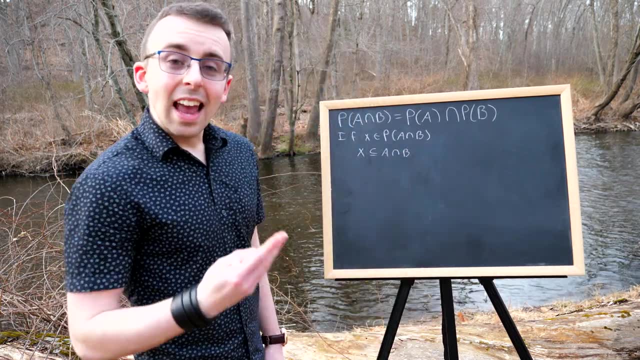 that x is a subset of A intersect B. By definition it's an element of the power set of A intersect B. So this means x is a subset of A intersect B. So that means every element of x is in A and every. 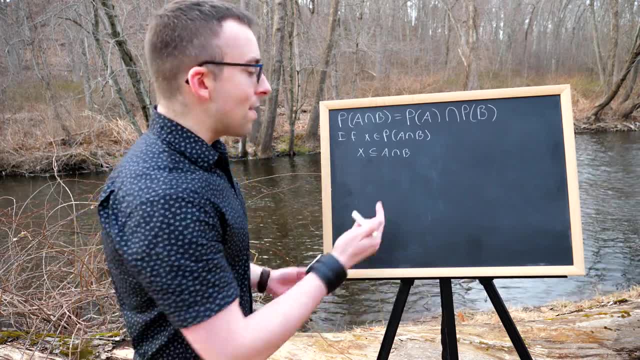 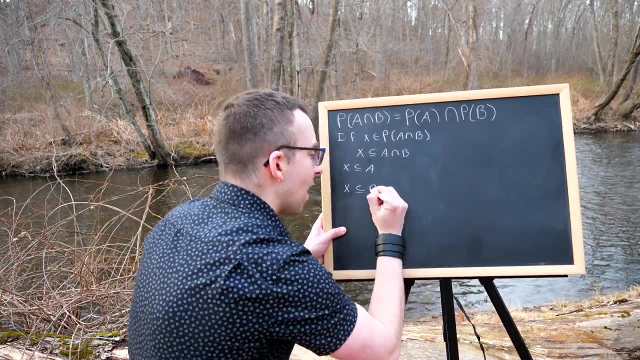 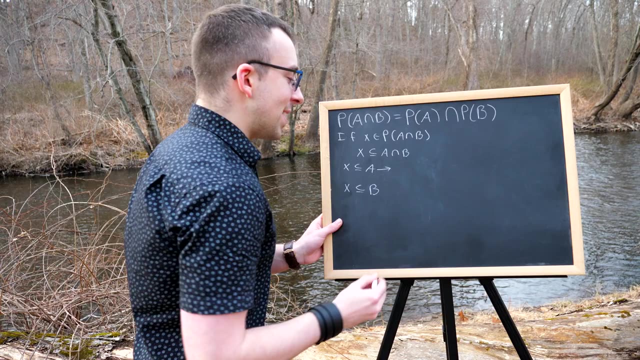 element of x is in B, which would mean that x is a subset of A. so we could write that here: x is a subset of B. Ah, now you see we're getting close. x is a subset of A. so what can we conclude? Well, by definition, that means: 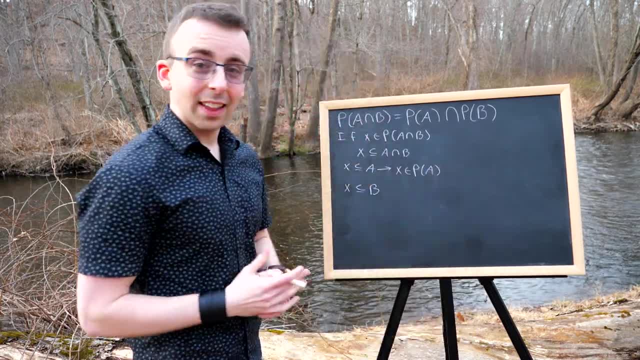 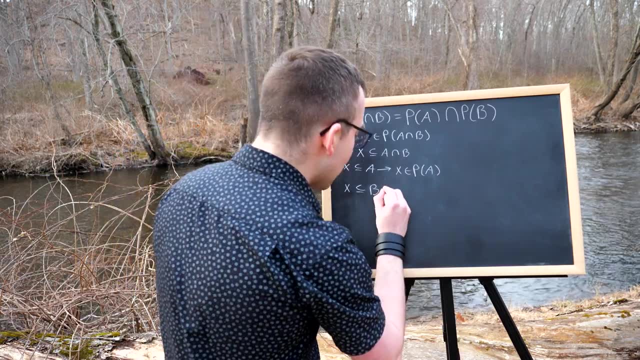 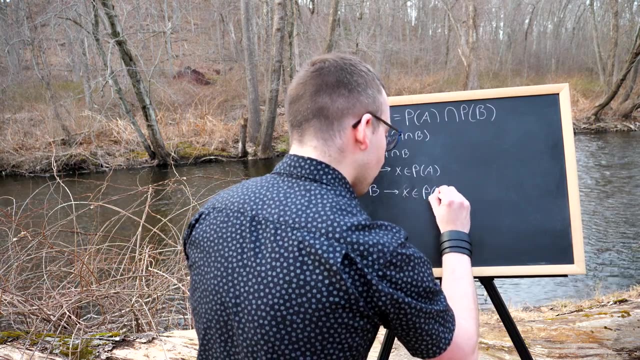 that x is an element of the power set of A, since the power set of A just contains all the subsets of A. Similarly, since x is a subset of B, we can conclude- whoops, that x is an element of the power set of B. So x is in the power set of A, x is in the power set of B, thus it's in their. 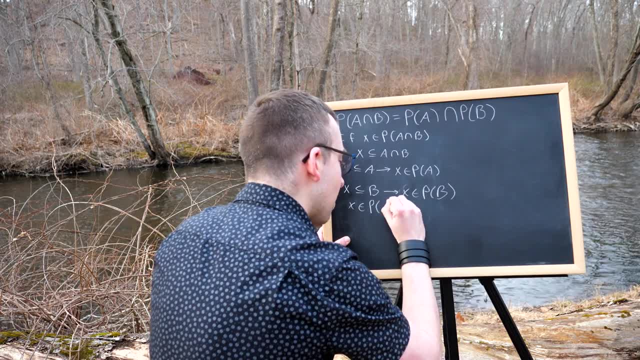 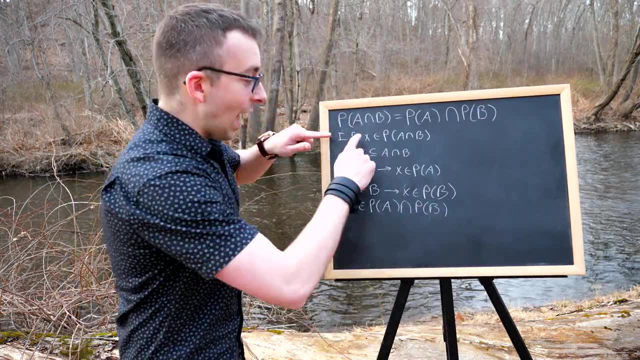 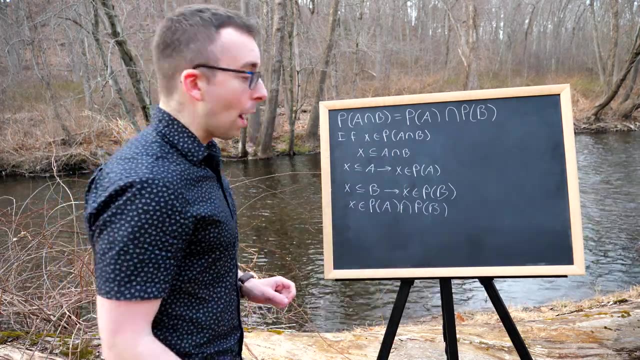 intersection x is an element of the power set of A intersected. now my chalk broke- intersected with the power set of B, And so we've proven that any element of the power set of A intersect B is also an element of the intersection of power set of A and power set of B. Thus, by 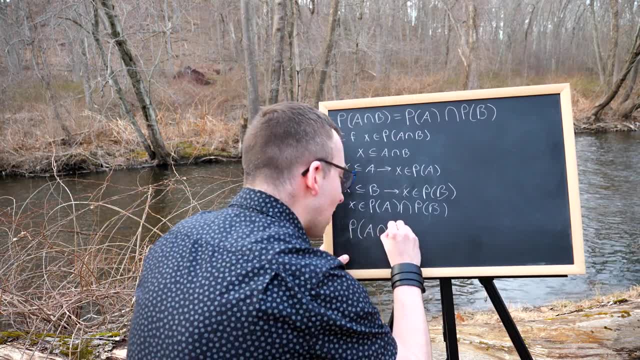 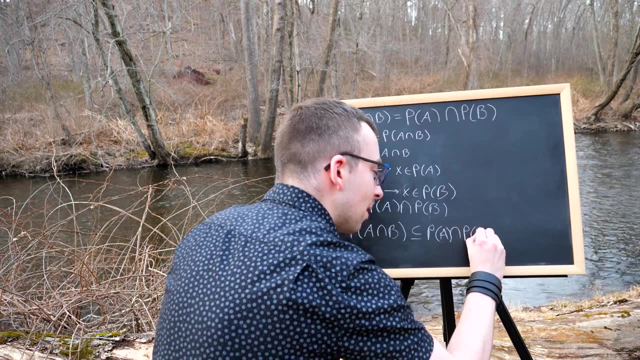 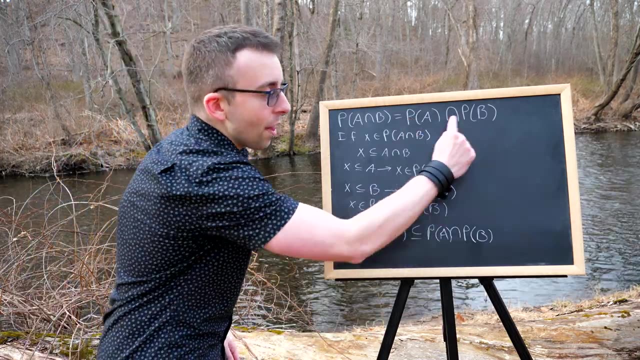 definition of subset. the power set of A intersect. B is a subset of the power set of A intersected with the power set of B. Sorry for a bit of sloppy writing there at the end. So all that remains for this set equality proof is to prove that x is a subset of B. 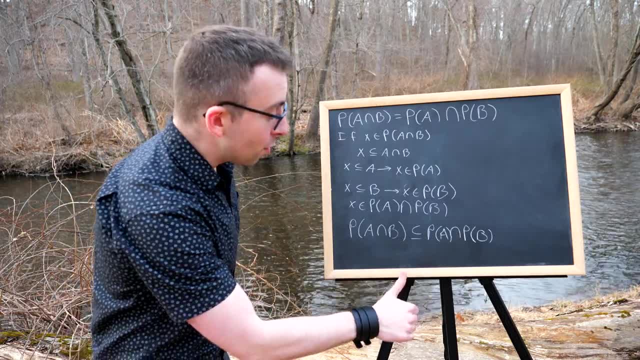 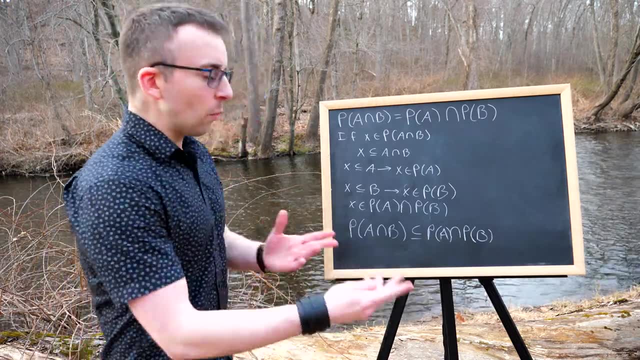 So this is a subset of this. Like I said, we can just do this going backwards. Maybe you could cover the screen now and try to do that yourself. I'll narrate you through it anyways. We would just begin with an arbitrary element of the power set of A intersected with the power set of B. 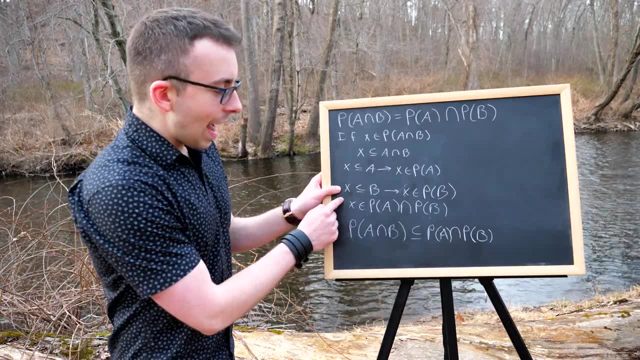 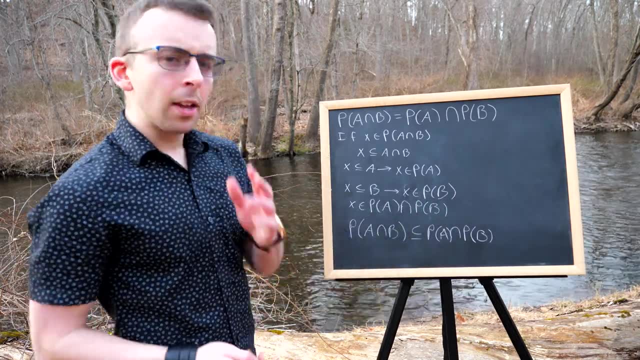 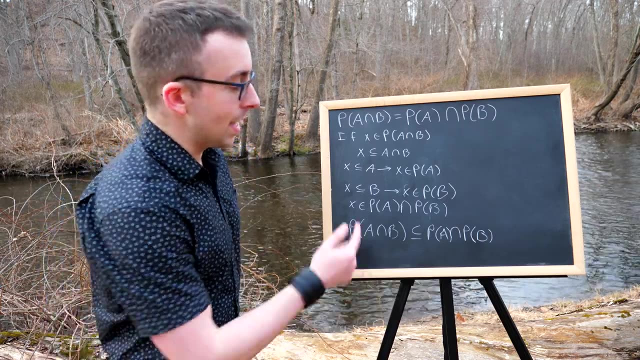 Then, being an element of that intersection means that x is an element of the power set of B over here and x is an element of the power set of A. By definition of power set, x must be the subset of A and x must be a subset of B, since it is in both their